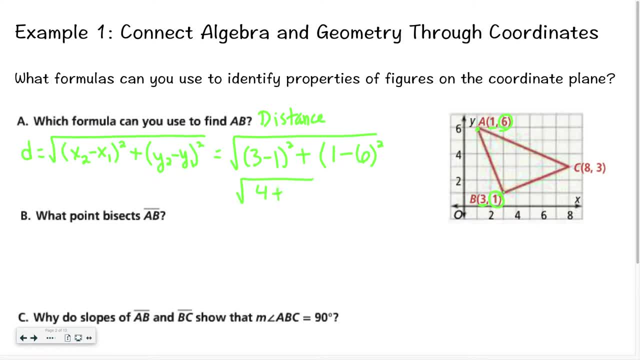 2 squared is 4.. 1 minus 6 is negative 5.. Negative 5 squared is 25.. That means That means That means Between them is the square root of 29.. Okay, Letter B: What point? bisects segment AB. 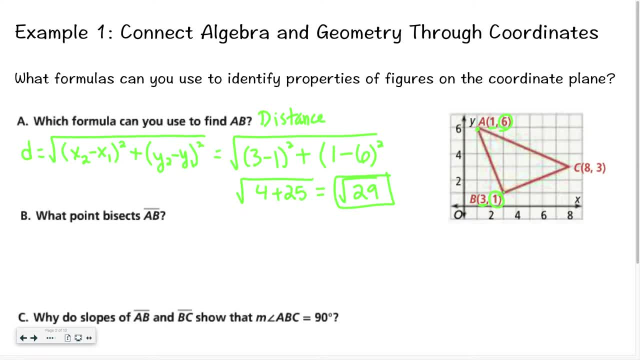 Remember, bisect means cut in half or halfway. So what's halfway between A and B? That means we're going to use our midpoint formula. So in order to find our midpoint, I'm going to add my x's together, So I have a 3 and a 1.. 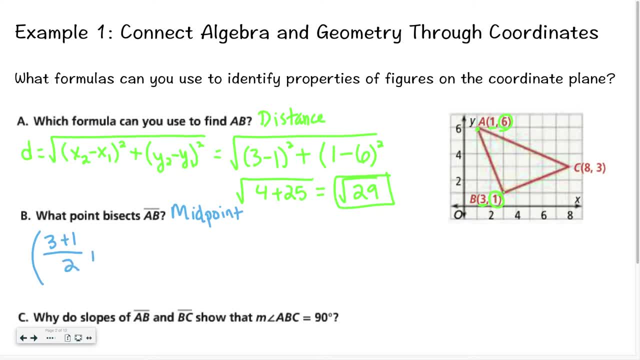 Divide by 2.. My y's 1 and 6.. So I'm going to say 1 plus 6.. Divide by 2.. So 3 plus 1 gives me 4.. 4 divided by 2 is 2.. 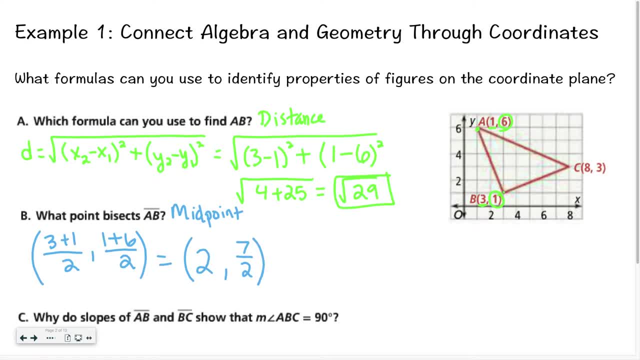 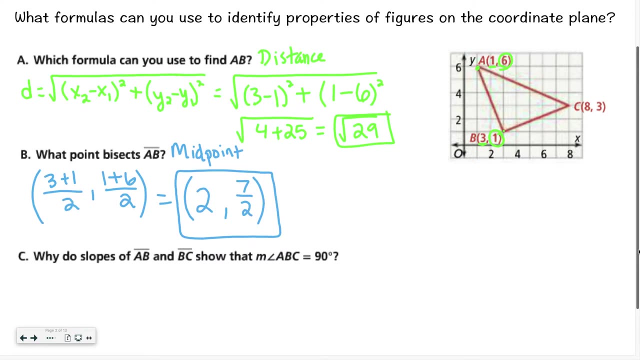 1 plus 6 is 7.. 7 divided by 2.. I'm just going to leave as a fraction, And that is the point that bisects AB. Okay So, distance formula, midpoint formula, Letter C: Why do slopes of segment AB and segment BC show that? 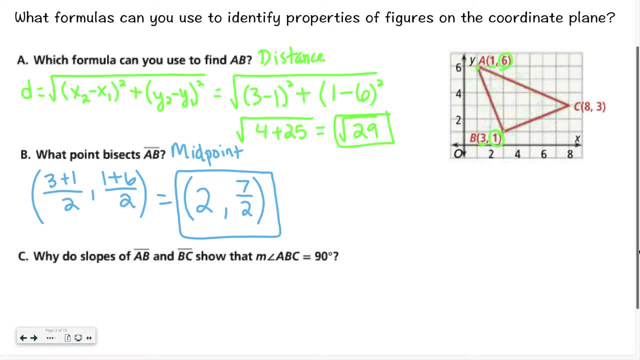 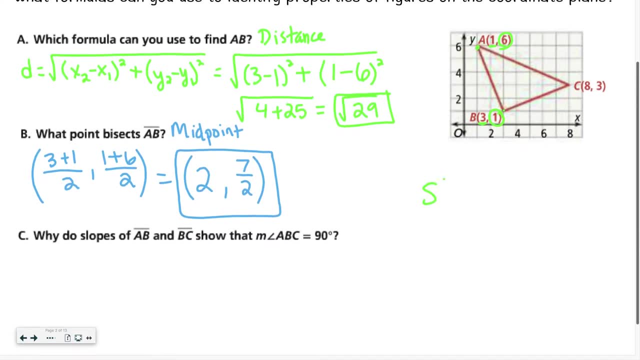 the measure of angle ABC equals 90 degrees. So slope- remember it's been a while Slope- is y2 minus y1 over x2 minus x1. And if they are 90 degrees that means our slopes are opposite reciprocals. 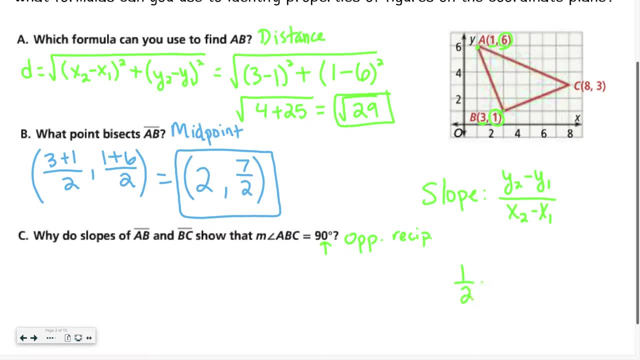 If you remember. So if I have a 1 half, my perpendicular slope is negative, 2 over 1.. So that's the situation we're looking for. Let's find the slope of segment AB. So I'm going to take my y value. 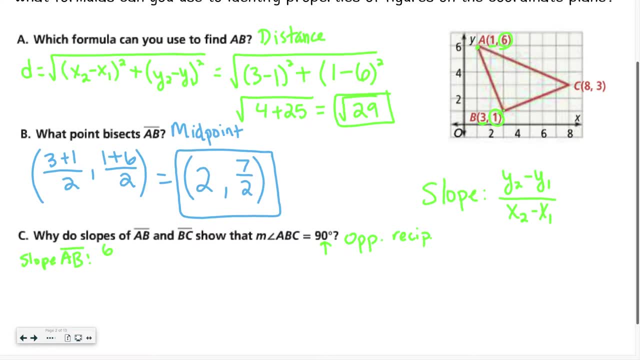 So if I start with 6 and then my other y value, I'm going to say minus 1.. Since I started up here at the 6 for the y, that means I have to start with the 1 for x. So I'm going to say 1 minus 3.. 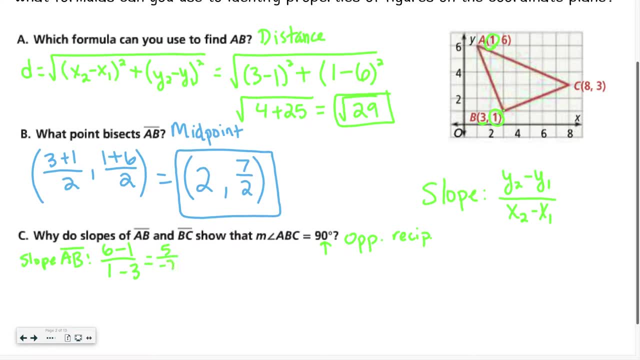 So 6 minus 1 is 5.. 1 minus 3 is negative, 2. That's the slope for AB. Now the slope for BC. Let's see. If I take the y value, I have a 3 minus 1 over 8 minus 3.. 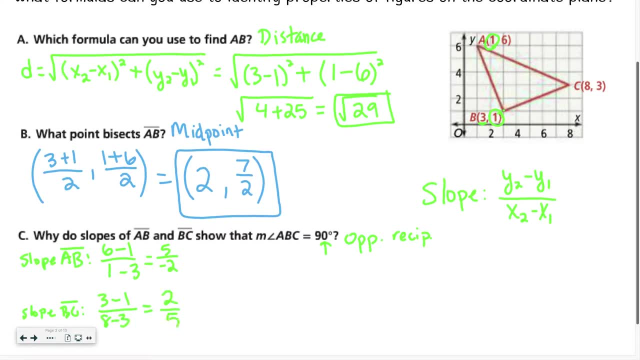 So 3 minus 1 is 2.. 8 minus 3 is 5.. So are these opposite reciprocals. So remember, reciprocal means that you take a fraction and you flip it. So in this case I started with 5 on top and 2 on bottom. 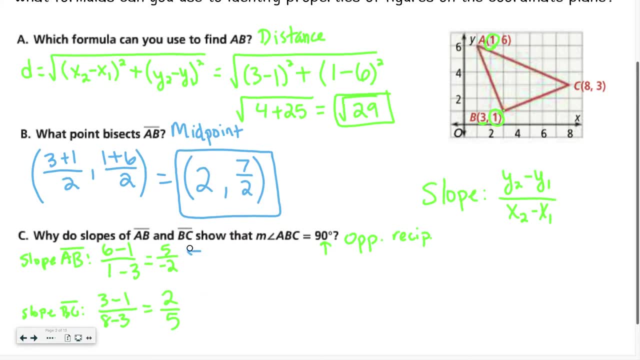 And then for the next one I had 2 on top and 5 on bottom, So they're reciprocals And opposite just means 1 is positive, 1 is negative. In this case they are. So the reason they show that it's a right angle. 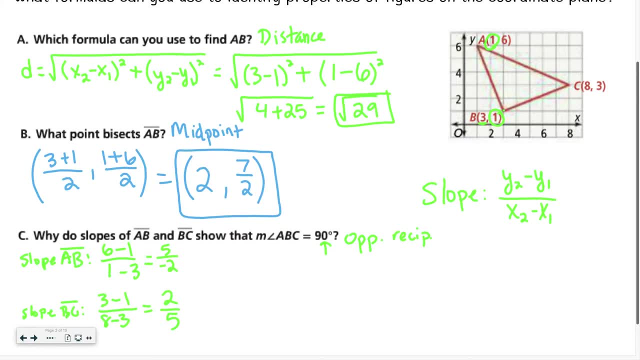 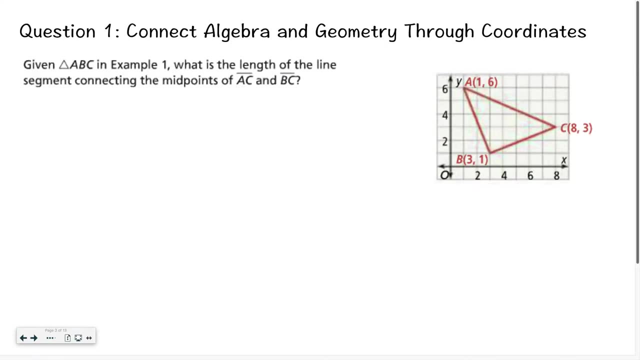 is because they have opposite reciprocal slopes. So there's all of your previous knowledge: Distance formula, midpoint formula and slope. Now we're going to use that repeatedly throughout this lesson. But why don't you look at this triangle ABC and find what is the length of the line segment? 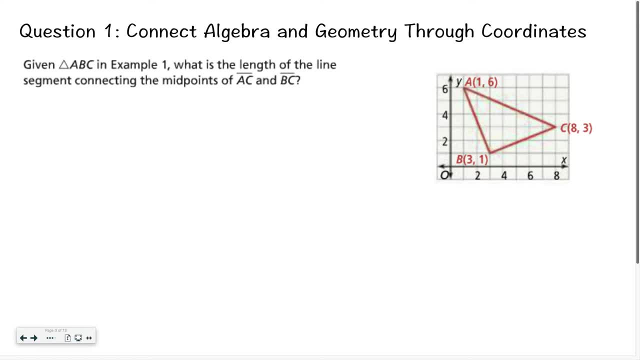 sorry, connecting the midpoints of segment AC and segment BC. So I want the length of the line. So that tells me I'm going to do distance, But I'm going to do distance with the midpoint. So first start by finding the midpoints. 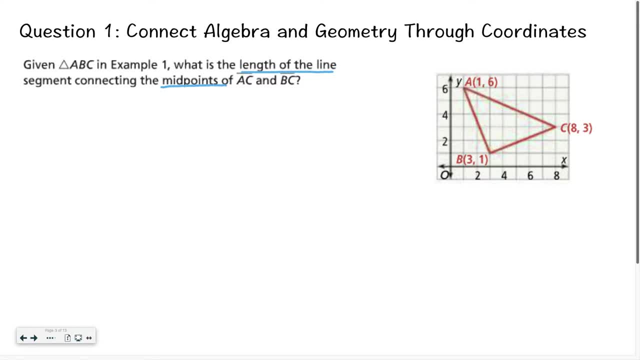 Then find the distance between the midpoints. Good luck. Hopefully, for your answer, you ended up with the square root of 7.25.. But if you did not get the square root of 7.25, and you said instead 2.69,, 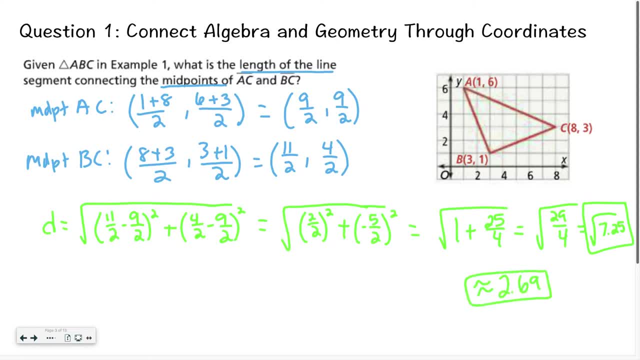 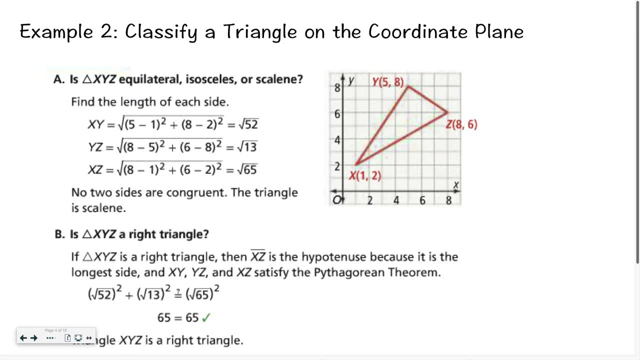 that is also a correct answer. Okay, Now let's talk about classifying a triangle on a coordinate plane. So if I want to figure out if something's equilateral, isosceles or scalene, that means I'm going to be doing the distance formula. 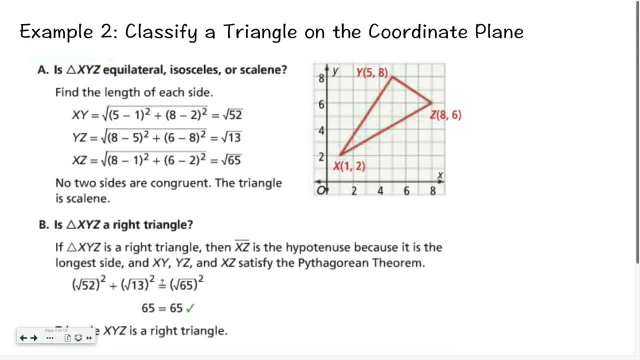 on each side of the figure in order to figure out if they have the same measures or different measures. Remember, equilateral triangles have three congruent sides, Isosceles have two congruent sides And scalene have no congruent sides. 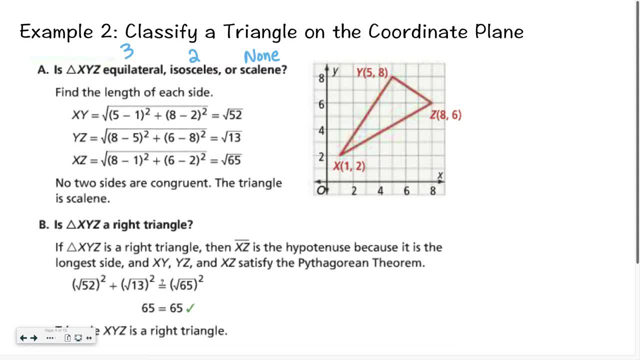 Okay, So I've already refreshed your memory on distance formula, So I decided I decided not to write it out again. The book did it for us. X, Y, they figured out, They found that it was the square root of 52,. 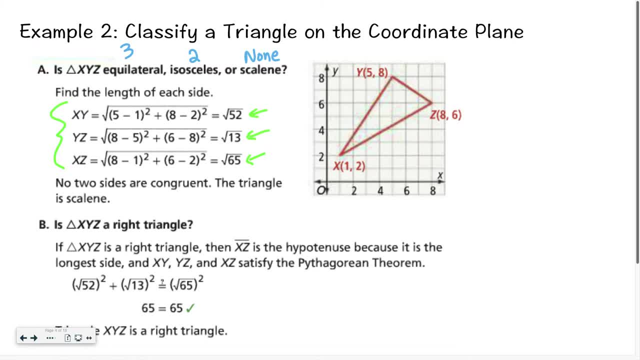 square root of 13, and square root of 65.. Since they're all different, the triangle is scalene. And then letter B. if I want to figure out if it's a right triangle, I mean you could go through and you could find all of the slopes. 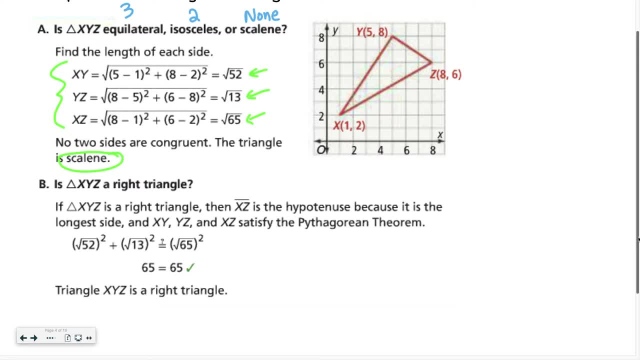 and see if you have any opposite reciprocals. But a faster way if you already know what the three measures are. we have Pythagorean theorem. I can say: the square root of 52 squared is: let's quickly refresh our memories on that. 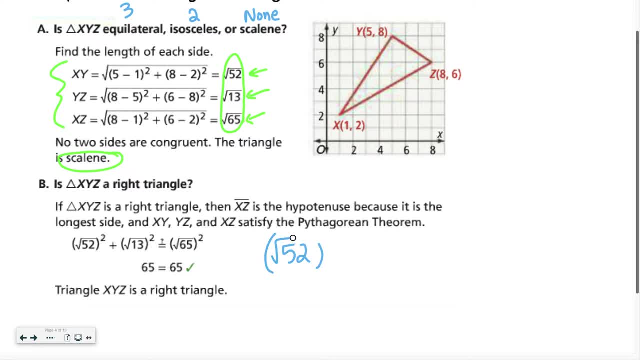 Remember, squares and square roots cancel each other, So then you're left with just whatever's under the square root, So in this case that's 52.. So then this ends up becoming 52 plus 13.. Does that equal 65?? 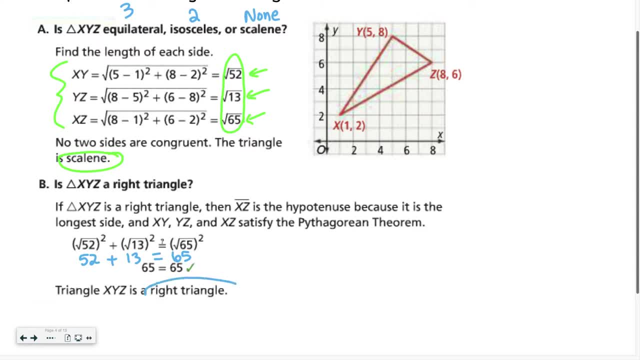 It does. So we know that this is a right triangle, and make sure that when you set up a Pythagorean theorem to try to figure out if it is a right triangle, the side that's the biggest always needs to be on its own. 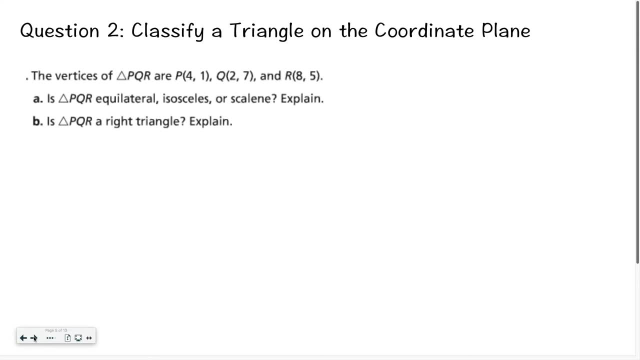 Why don't you go ahead and solve this next one? Good luck, All right For this problem. hopefully you ended up with two sides that were the same length, So you knew that they were, or that this forms an isosceles triangle. 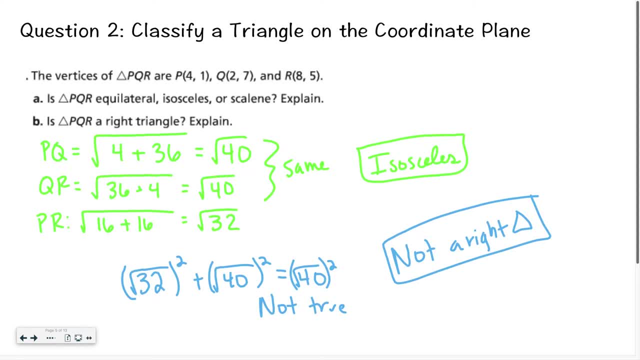 And you figured out, if you do Pythagorean theorem, it doesn't work because our two congruent sides happen to also be the longest sides. So we would say that they are not. they don't form a right triangle. Another quick side note. 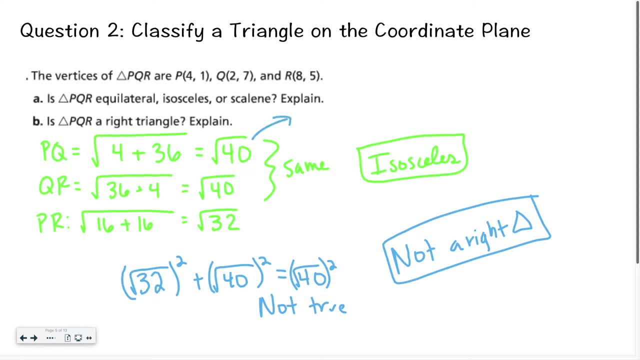 this is another chapter where we're going to practice simplifying radicals. So the square root of 40, I could split up into the square root of four times the square root of 10,, which becomes two square roots. So I could split up into the square root of 10,. 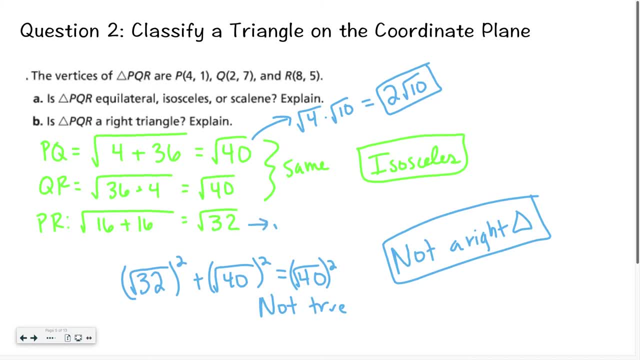 just like 32, I could split up into the square root of four times the square root of, or actually the square root of 16 times the square root of two, which becomes four square root of two. Okay, So you will have to practice that this chapter. 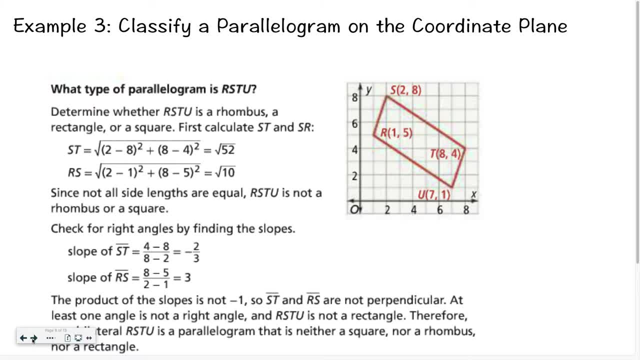 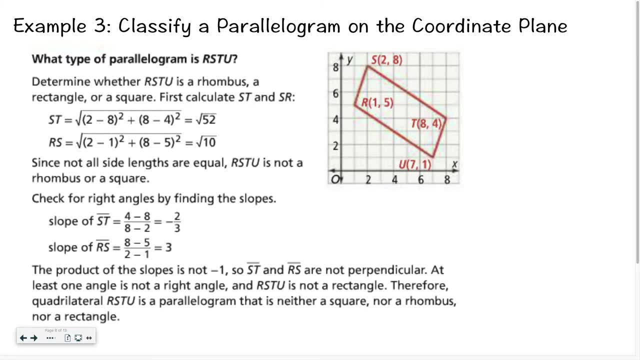 All right. Example three: let's talk about classifying a parallelogram on a coordinate plane. So if I want to figure out what type of parallelogram is, uh, RSTU. so remember, parallelograms are kind of. 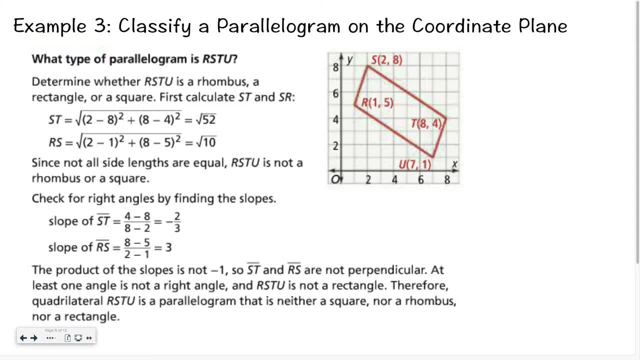 um, the biggest category of quadrilaterals that have two opposite sides, or two sets of opposite sides that are parallel, Um parallelograms. then, more specifically, it becomes rectangle and rhombus, And then, if it's all of those, 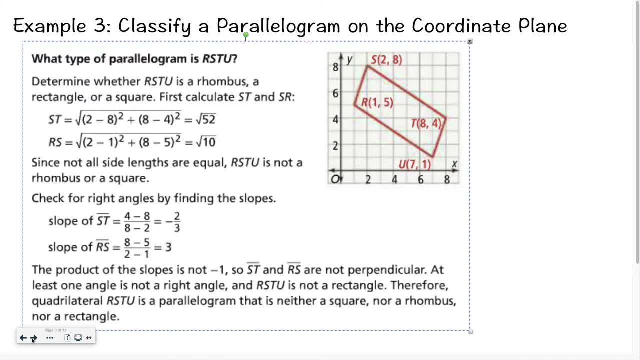 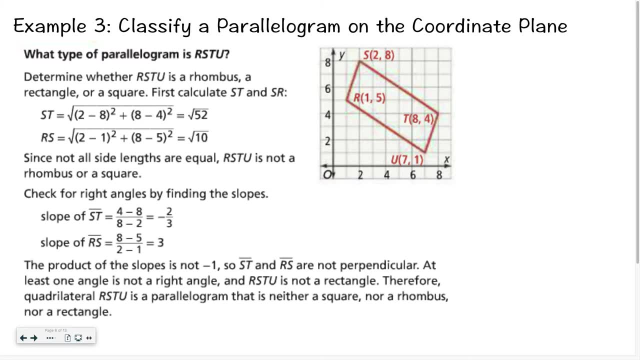 it is a square, So we're going to go through the process to see what figure do we have? Okay, So what type of parallelogram is RSTU? So first we have to find the distances, and you don't have to do it on all four sides. 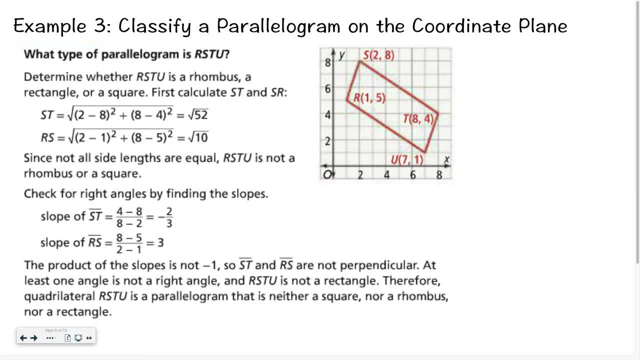 because if we know it's a parallelogram, we know we have two sets of congruent sides. So that means I would only have to do it on um- let's see RS, because that's the same as UT, or I would. 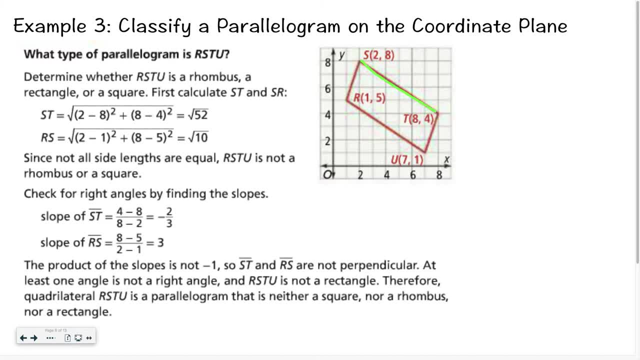 or sorry, and I would have to do it on either side. I would have to do it on either ST or RU, because those are the same. So if I do that distance formula, I get square root of 52 and square root of 10.. 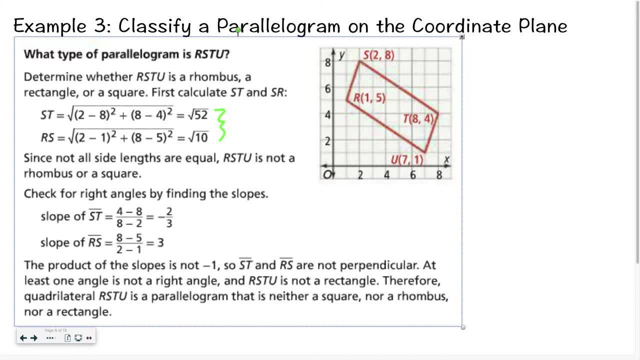 And then, since not all side lengths are equal, RSTU is not a rhombus or square because remember rhombi and squares have all four sides are congruent. So if you got the same measure for both sides immediately you're going to think maybe it's a rhombus or square. 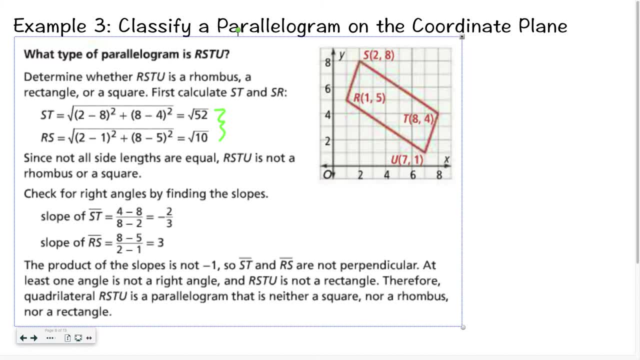 But now we know that it's not a rhombus, not a square. So that leaves us with parallelogram or rectangle. So in order to know if it's a rectangle, what I can test is the slopes of the sides to see if I have right angles. 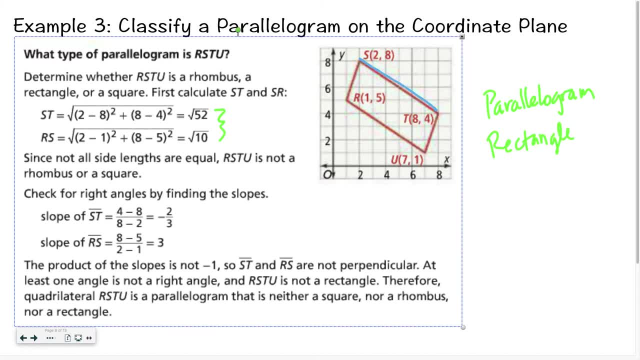 So if I find the slope of ST and I compare it to one of the shorter sides, if it's a right, if it's a rectangle, there'll be opposite, reciprocal slopes. So if I find the slope of ST, I end up with negative two thirds. 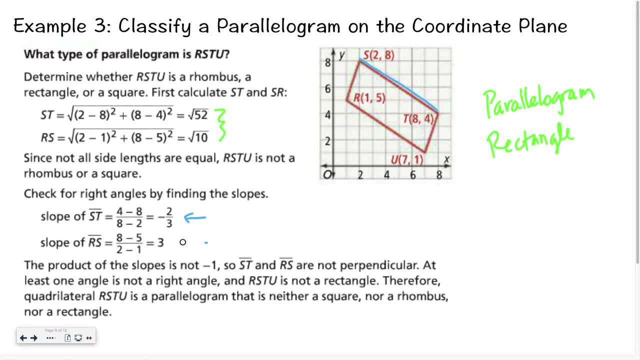 If I find the slope of RS, I end up with three. Those are not opposite reciprocals, Therefore they do not form 90 degree angles. So I can rule out rectangle And that means that this is just a parallelogram and not a rectangle, rhombus or square. 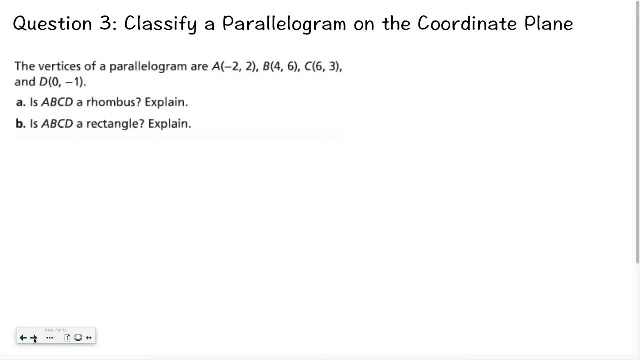 Why don't you go ahead and take a look at this problem on your own? Good luck, All right. Hopefully for this question you figured out. it's not a rhombus because we do not have congruent sides, But it is a rectangle because if we check the slopes, 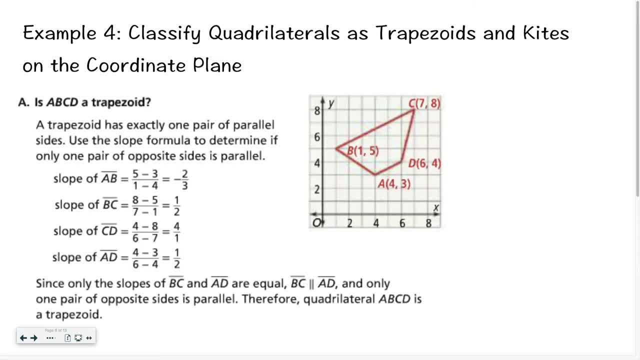 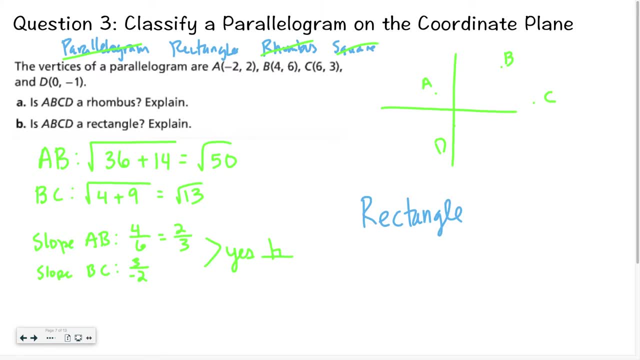 we have opposite reciprocals, So they form right angles, All right. One last thing on that question. I recommend, if you're ever just given vertices, maybe try just even a rough sketch of plotting them out So you have a nice visual. 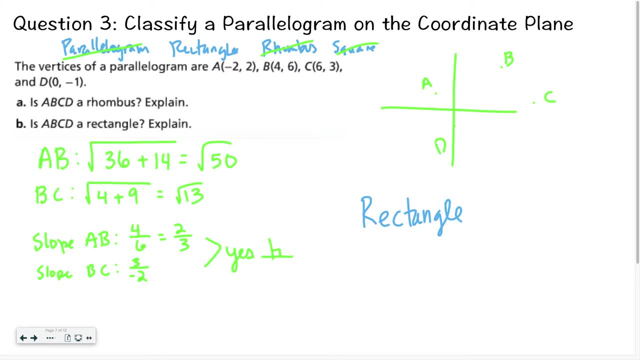 So you end up choosing the correct sides. Sometimes I see students that, without the visual, they end up trying to compare AB to DC And then they're like, Oh cool, I have congruent sides. So that means that this is a rectangle or this is a rhombus or a square. 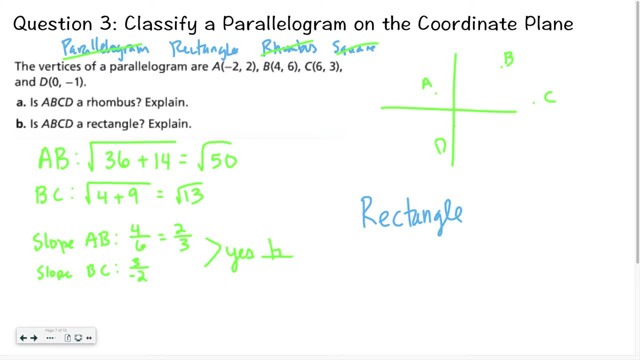 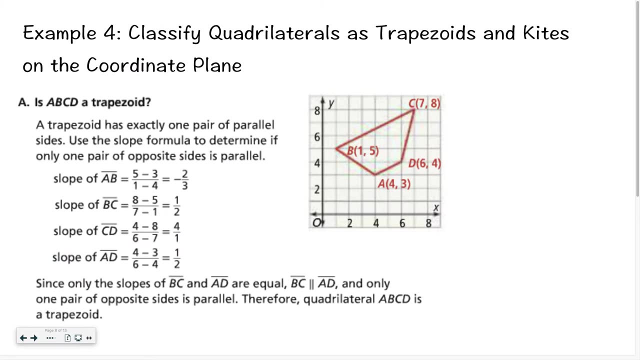 but that they got false information because they chose opposite sides which are always going to be congruent in a parallelogram. Okay, So example four: What if we want to check for a trapezoid or kite? So you're still using the same tests. 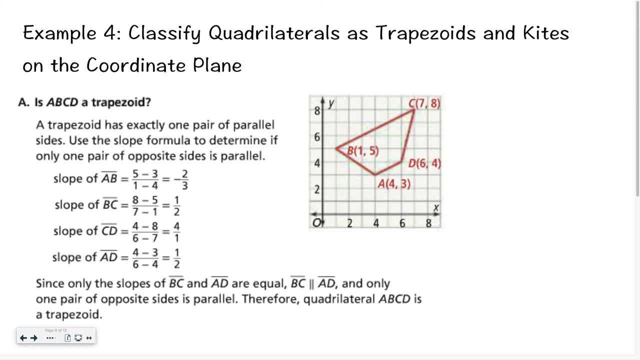 Remember, a trapezoid has exactly one pair of parallel sides, So we've talked about perpendicular slope. Parallel slope is when they're exactly the same. Okay, So that means to check for a trapezoid. you do the slope of all four sides. 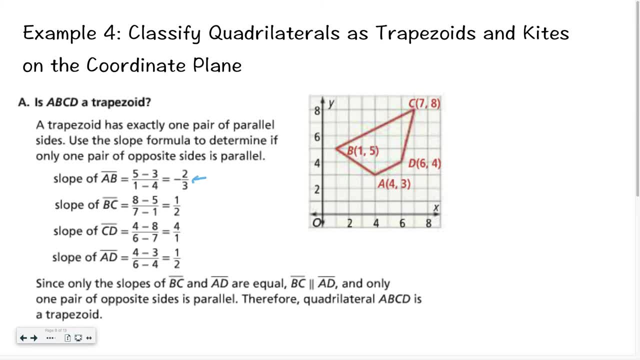 So they found the slope of AB was negative two thirds, BC was one half, CD was four And AD was one half. So, if you notice, we have two sides that are parallel to each other And since we have one set of parallel sides, 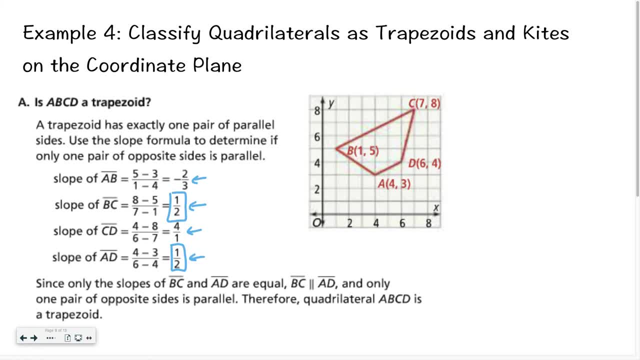 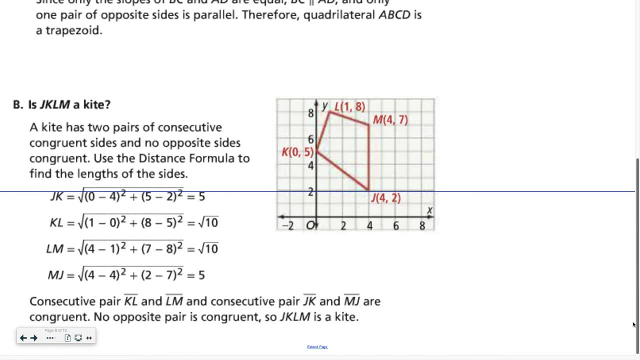 that means that this is a trapezoid. That is all you have to do to check for a trapezoid. Okay, And then if we want to know if something's a kite, the way you do that is. a kite has two pairs of consecutive congruent sides. 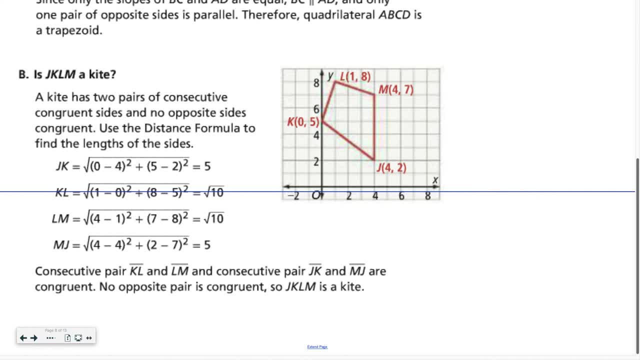 and no opposite sides. So for a kite, you're going to use the distance formula to find the distance of all four sides And you can see right away. okay, I have two sets of congruent sides, but the key part of making this a kite is they have to be right next to each other. 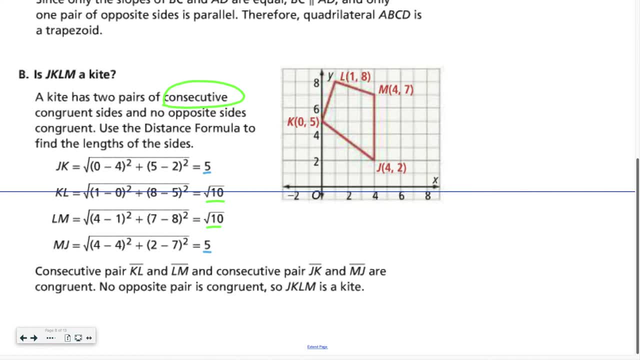 So, again, this is where drawing a rough sketch of where those points are really helps. So KL needs to be congruent to LM, And it is. They're both the square root of 10.. And same thing goes for KJ and MJ. 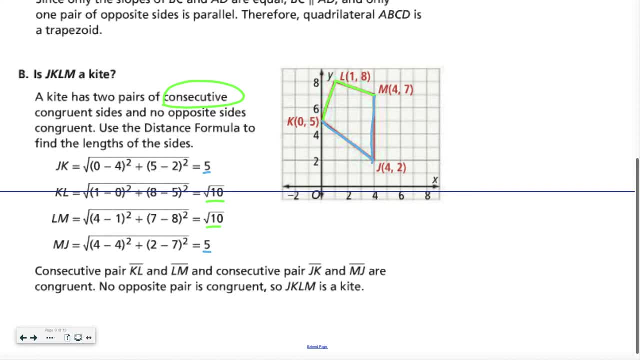 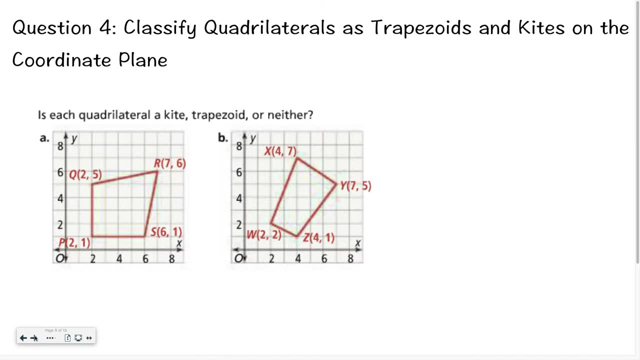 Both need to be congruent as well, And since they are, that means that we have a kite. So I think you guys have seen the pattern by now. You're doing a lot of distance formula slope, You're doing a lot of midpoints. 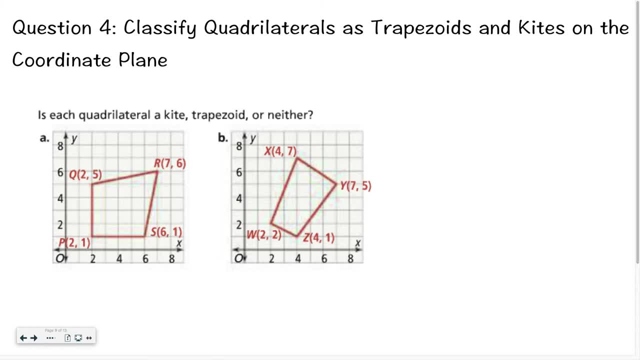 It's a lot of the same thing. And then just knowing what makes something a parallelogram, rectangle, rhombus, square, kite, trapezoid, all of those things- So I want you to check to see is either quadrilateral? 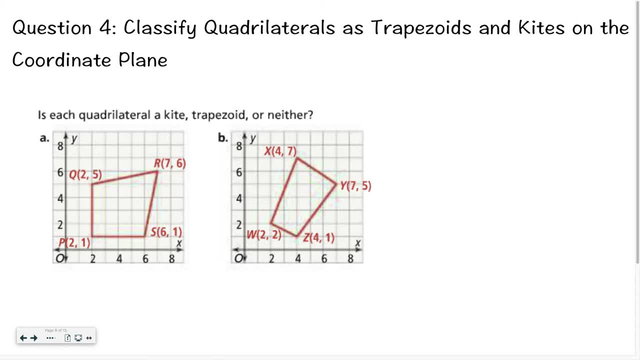 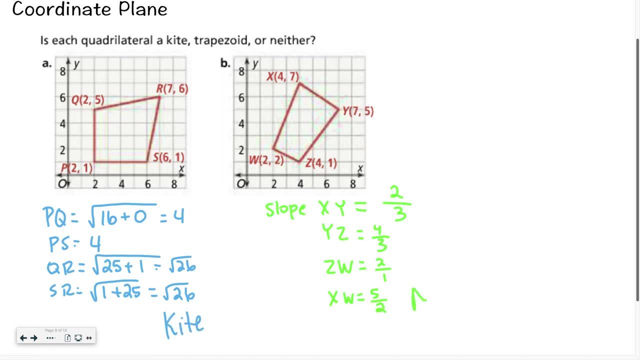 a kite, trapezoid or neither. All right, Hopefully for this problem. you said that letter A is a kite because you have two sets of consecutive sides that are congruent, And then letter B is actually neither. So if you find the slope, 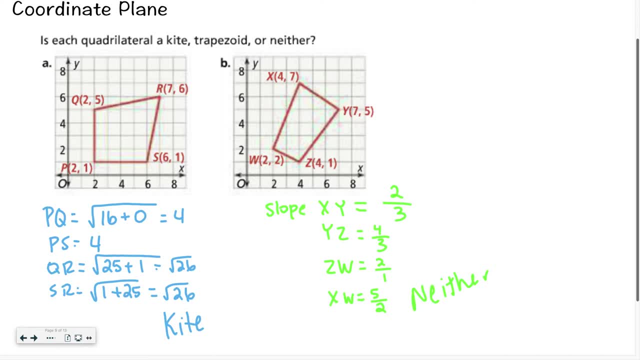 none of the slopes are parallel, And also if you look at the sides, you can see that we don't really have two sets of congruent sides going on either. So I totally- just from a visual standpoint- skipped the kite test for that one. 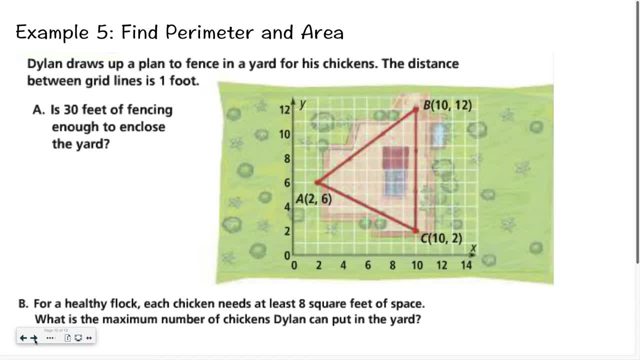 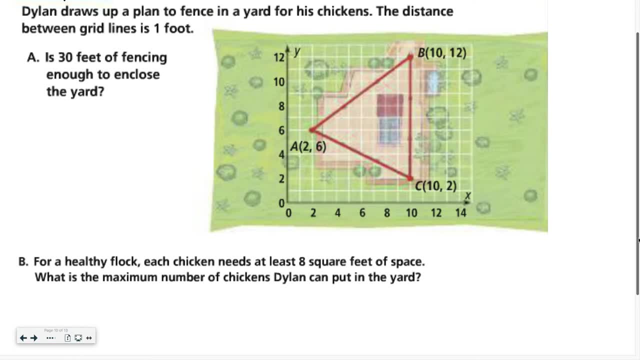 Okay, Example five. So I'm not going to go through and actually solve this, I just want to talk you through how you would solve it. So if we look at this example, we're talking about finding perimeter and area. So Dylan draws up a plan to fence in a yard for his chickens. 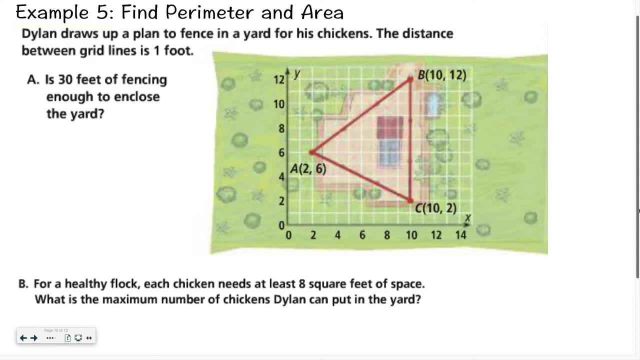 The distance between grid lines is one foot. So we want to know: is 30 feet of fencing enough to enclose the yard? The way that we would figure that problem out is we would find the distance of all three sides and we would add them together. 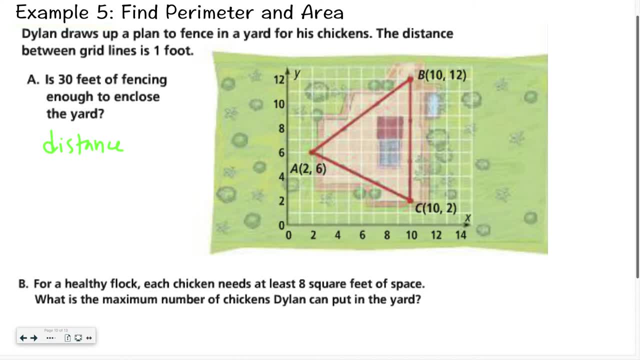 And we would see. if I take the lengths of all three sides, add it together, is it less than 30?? If it is, I have enough fencing. If it's not less than 30, then I need more fencing or Dylan needs more fencing. 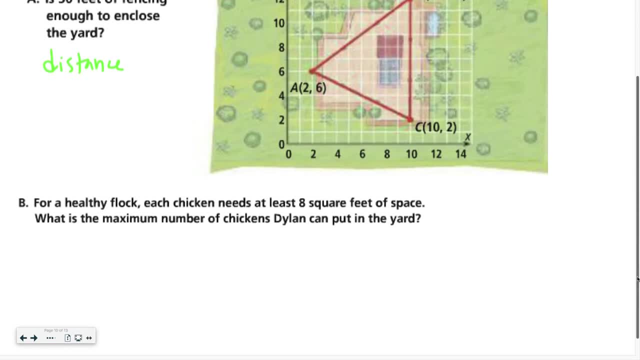 I guess The more complicated problem in this example is finding the area. So to find the area of a triangle you guys know is one half base times height. You guys have been working with that for a really long time by now. 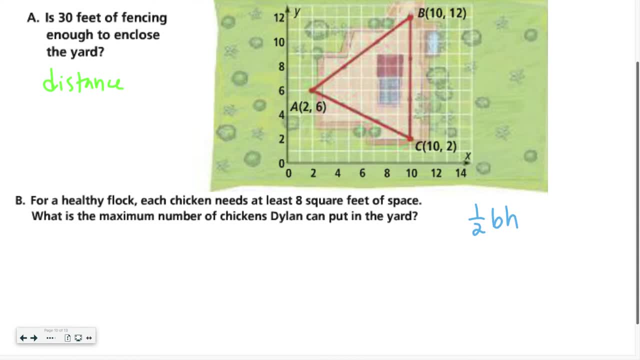 And the really important thing to know about finding the area on this triangle is if? well, first of all, if I had already done letter A, I would know that AB is 10,, I would know that BC is 10,. and then this other side. 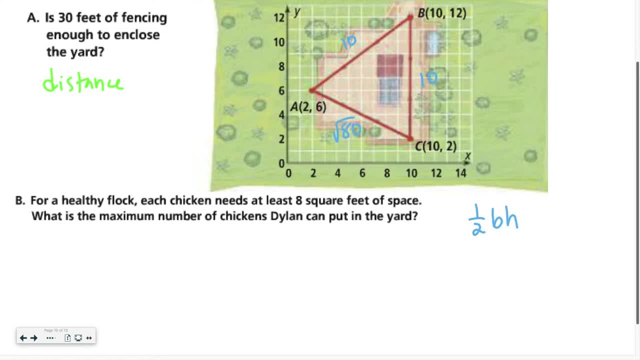 I would have found is the square root of 80.. Okay, so that's what I would have found in letter A, Letter B. now what I would use is: I need to find the height of this triangle. Remember, height of a triangle always has to come from a right angle. 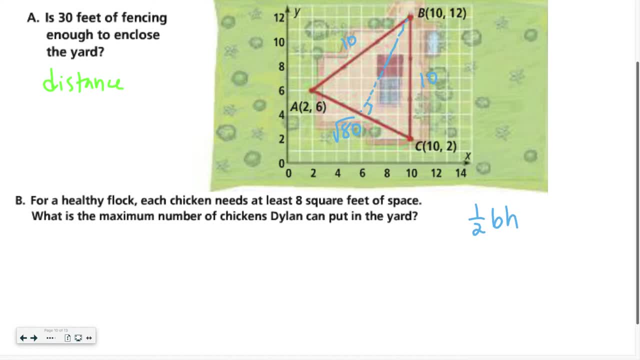 It has to come from an altitude. So we have to find what that distance is. So that means I have to find the midpoint of AC. So if I found the midpoint of AC I would say 2 plus 10 is 12,. 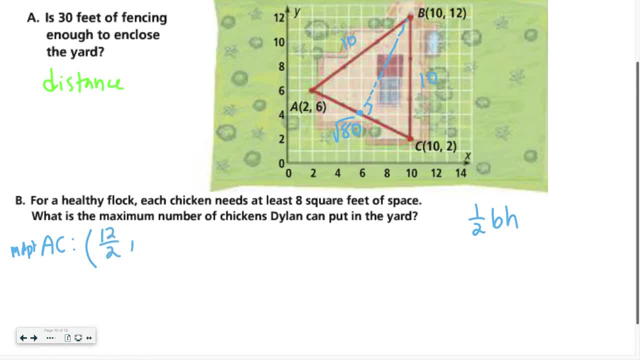 divided by 2.. And then I would say: 6 plus 2 is 8, divided by 2.. So my midpoint is at 64. And then what I would do is I would find the distance between my midpoint.